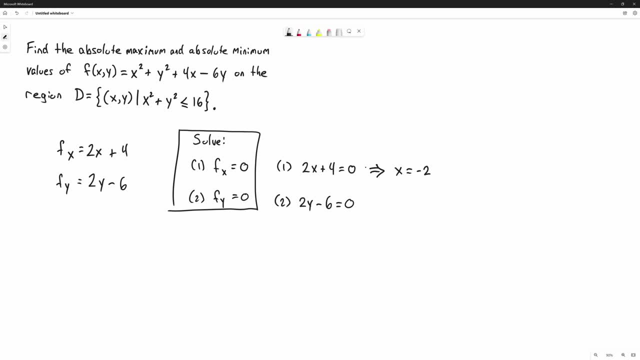 Since that is the only condition. coming from equation 1,, that means that we have an x coordinate of negative 2.. The other equation must give us the y coordinate. So if you solve equation 2, it'll give you a y coordinate or y value of 3.. 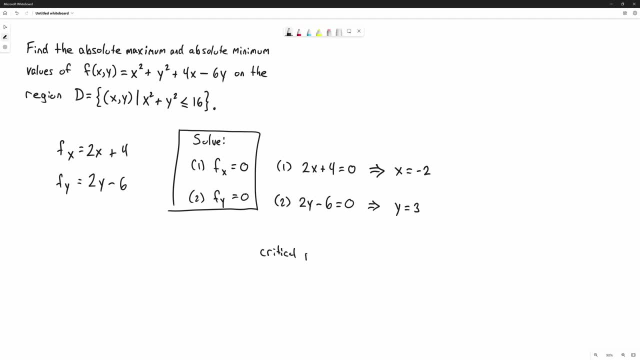 So if you go ahead and put that together, you get a single critical point with coordinates negative 2 comma 3. Now it's worth checking if that critical point is within the region and that underlined part there. the condition: all x comma, y values to which x squared plus y squared is less. 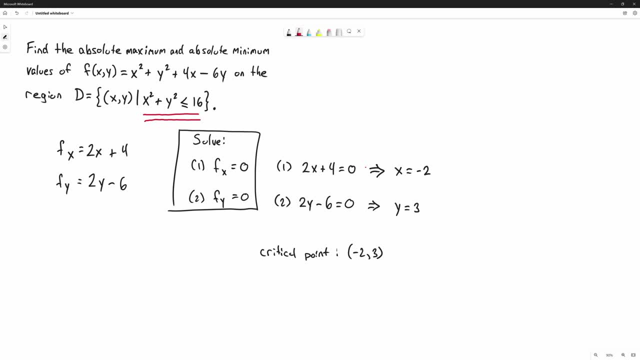 than or equal to 16, that's basically describing a region, that is a disk of radius not 16, but radius 4.. So if you go ahead and check, take your x coordinate square that, add that to the y coordinate, which is 3, plug that in, simplify that looks like you're going to get that. 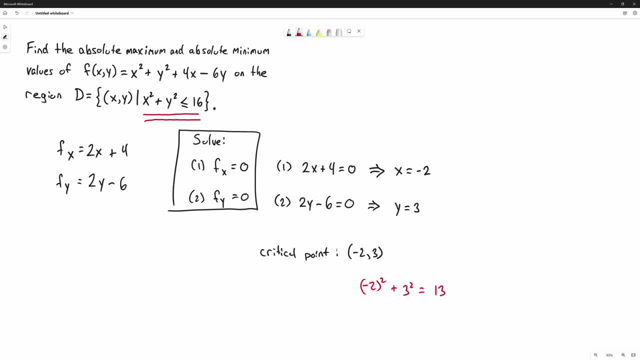 comes out to 13,, which is less than or equal to 16.. So that critical point is in the region. Now we have the critical point. We're going to want to plug that into the function that we're given, the function of two. 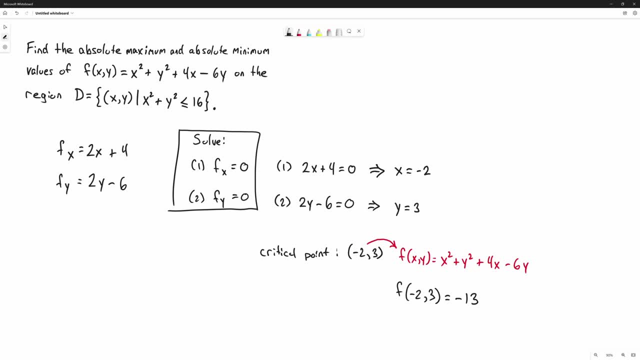 variables to check the value that we get at that critical point. So if you go ahead and plug in x is negative 2 and y is 3 to the function that we're given, that should come out to negative 13.. And that is one of our function values that we'll be comparing with later. 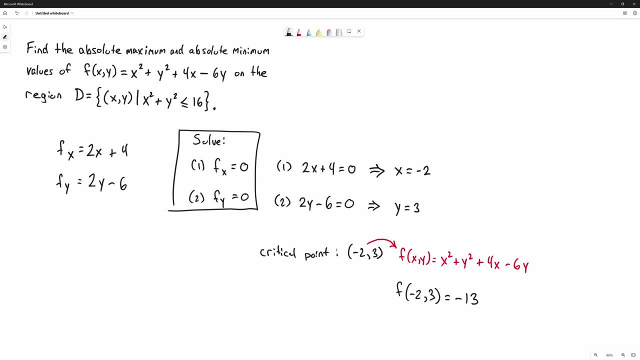 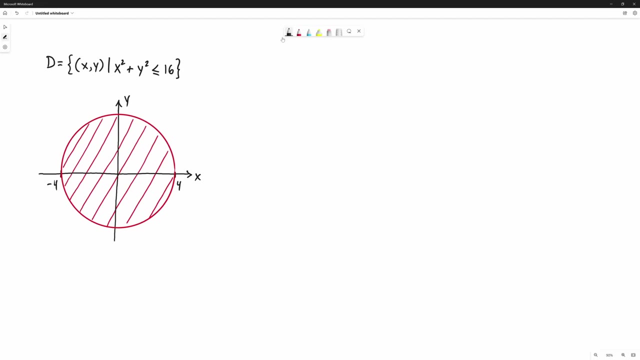 once we start checking the values of the function on the boundary of the region- And let's go ahead and get to that- describing the boundary, the region, and checking the values of the function on the edges or boundary To describe the boundary of our region- we're going to start by noticing that x squared plus. 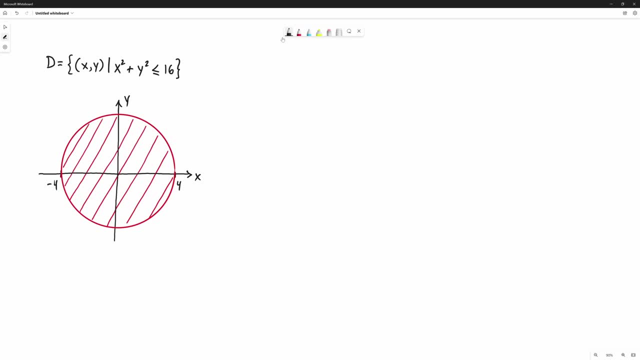 y squared less than or equal to 16, that basically is almost the equation of the circle. So what we're going to basically do is split this into an upper portion, and we'll call that curve one, and we'll split that into a lower portion and we'll call that curve two. Now, the edge, the circle, that's going to be the equation x squared. 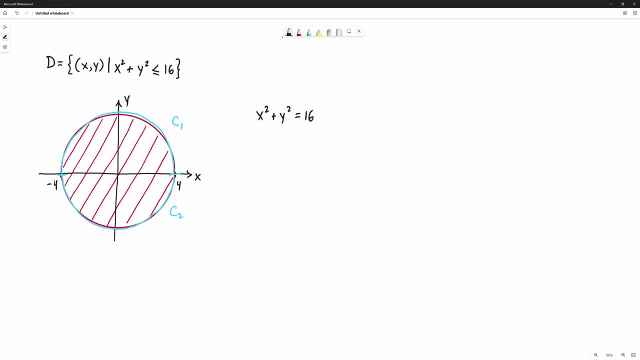 plus y squared equals 16, and to describe that y is a function of x, we can solve for y. So first go ahead and subtract x squared and then here take a square root- don't forget the plus or minus- and we get: y equals plus or minus the square root of 16, minus x squared. 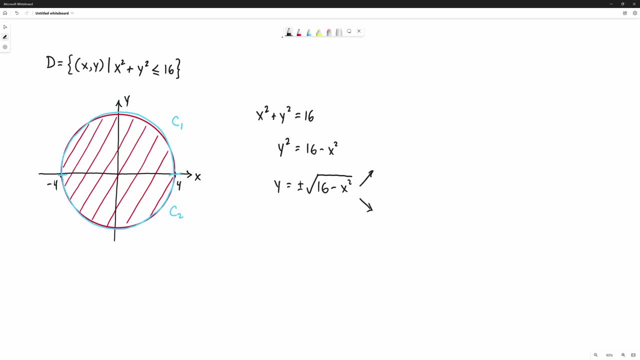 Now that's going to split into two parts: The positive root, that's going to give you the upper portion that we're going to use and call that c1, and the negative root gives you the lower portion, which we'll call that, corresponding to the curve c2.. 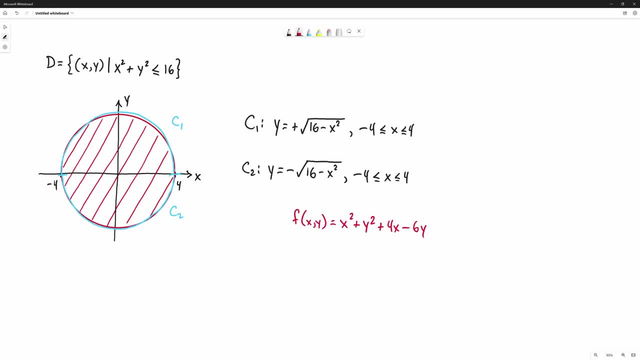 Now that we've described the boundary or edge of our region as two separate curves- y is a function of x- we're going to take each of those equations for y on curve one and curve two and individually plug them into our function of two variables and that's going to give us a calc one. 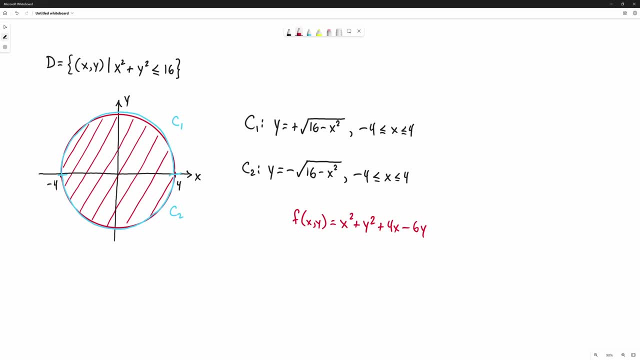 absolute max and min value problem. So let's go ahead and start by plugging in curve one where y equals the square root of 16 minus x squared. All right, let's take our time and simplify by plugging in y as the square root of 16 minus x. 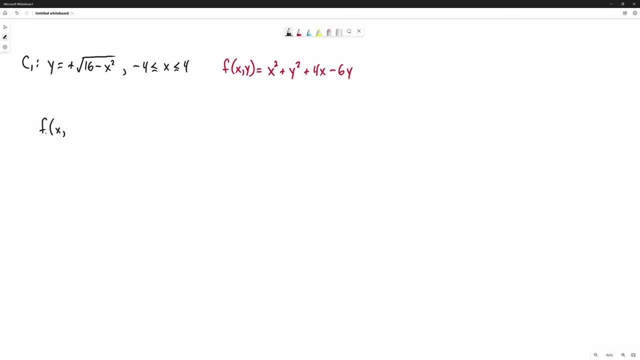 squared. So we're not plugging in anything for x, but in the y variable the input for y, we're replacing that and plugging it in with the square root of 16 minus x squared. So it looks like if you simplify that you'll get x squared and then the square root expression. 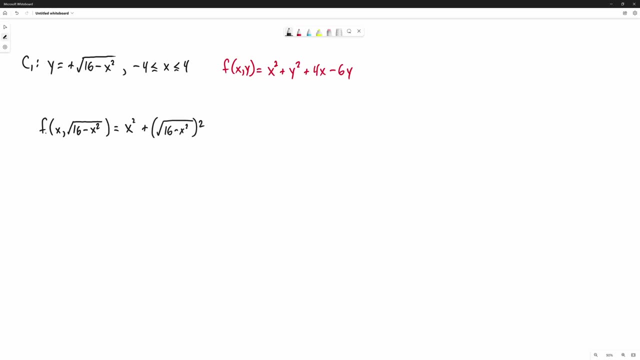 but that's going to be x squared, It's going to be squared and then plus 4x and then minus 6 times that square root expression. All right, and that's going to simplify nicely. the square is going to get rid of the square root. 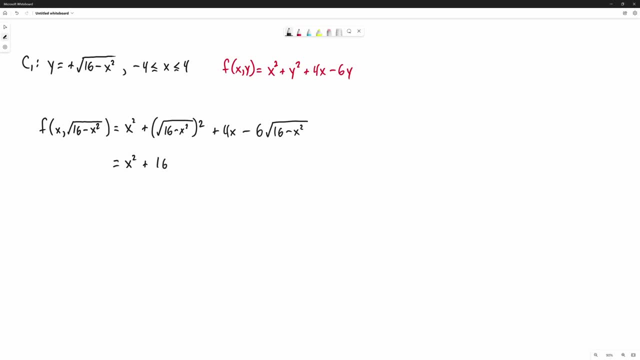 so you'll be left with x squared plus 16, minus x squared plus 4x, and then minus 6 times the square root, and it looks like we're going to be left with x squared plus 16, minus x squared plus 4x, and then minus 6 times the square root. 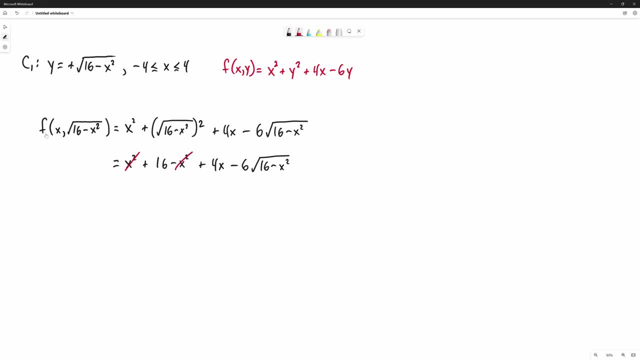 and it looks like you can cancel out the x squareds and get a pretty nice looking formula for the boundary value of the function on curve 1.. So it looks like we can write that as 16 plus 4x and then minus 6 times the square root. 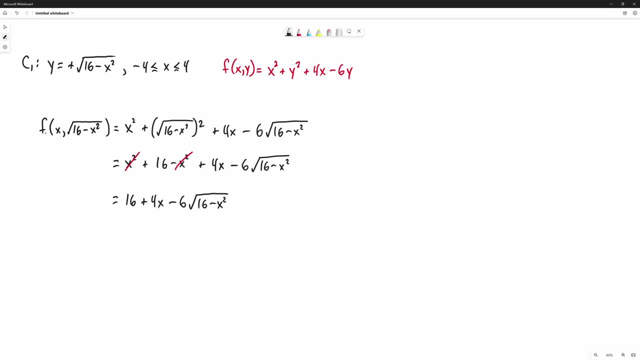 All right, and from here this now turns into a calc 1 problem. We're going to want to take this function of one variable. Notice that only depends on x, There is no y in it, And we're going to want to check. 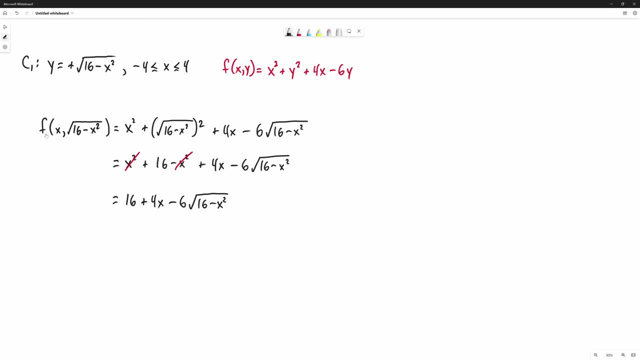 what the absolute max and min values are of that function on the interval of x values between negative 4 and 4.. To find the critical points of this function of one variable, we're going to start by finding the derivative, And it looks like here: 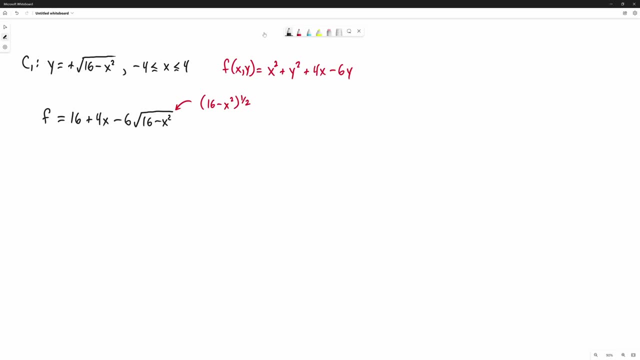 we're going to end up using the chain rule. Think of that square root as 16 minus x, squared all the way to the left, All to the one half power. So it looks like for the derivative that's going to come out to 4.. 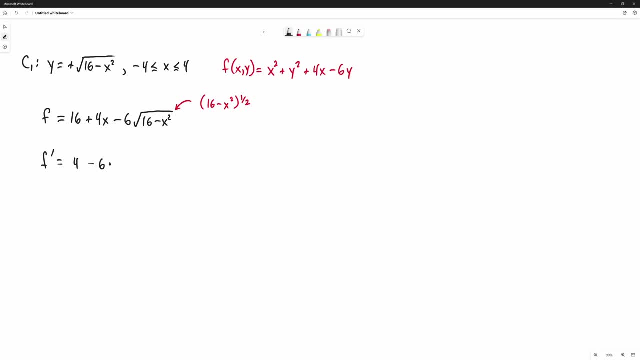 The negative 6 is just a constant. Apply the chain rule. bring the one half down. We're going to keep the inside the same. Subtract 1 from the power. one half Half minus 1 will give negative one half. And now we multiply by the derivative of the inside. 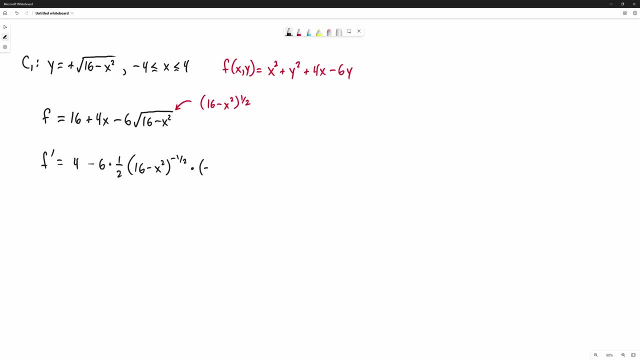 the inside being 16 minus minus x squared, The derivative of that is going to be negative 2x. All right, Now to solve for where that equals zero becomes undefined. you're going to want to simplify this, So it looks like you can cancel out a factor of two. 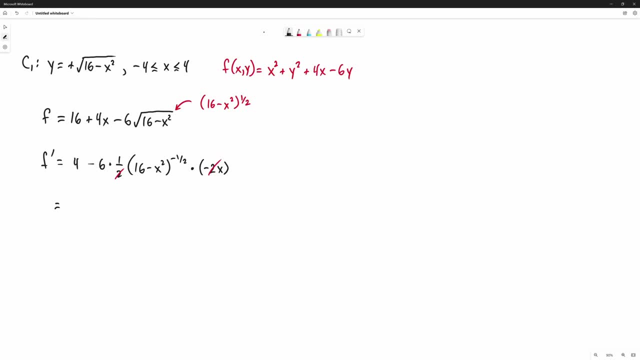 There is a negative that cancels out there. So it looks like we can write that as four And then plus the two negatives cancel. It looks like we have a factor of two. It looks like we have a factor of two. It looks like we have a factor of six, x. 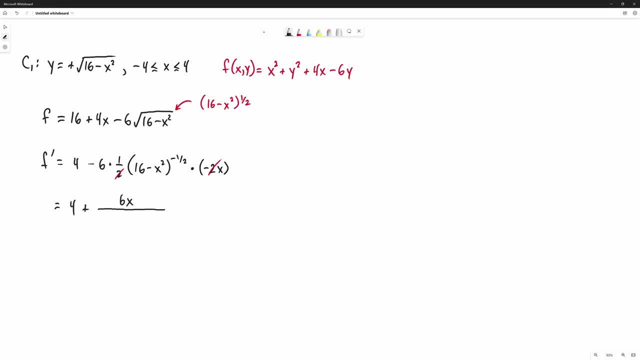 All the quantities with a positive exponent go in the numerator And I can write that negative one- half power- as a square root in the denominator. All right, And from here we're going to want to look for the critical points by setting that equal to zero and seeing what values of x. 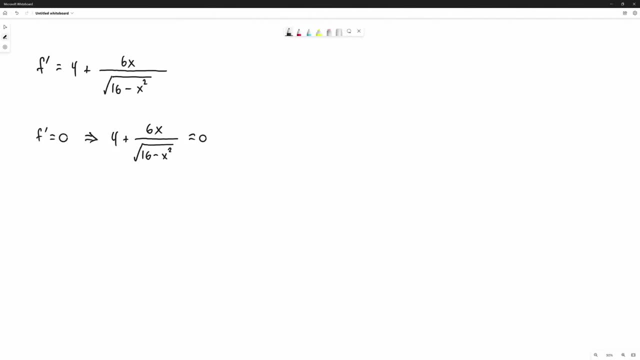 possibly make that undefined, All right. If we start by setting the derivative equal to zero to find the critical points, we get this equation: a combination of radicals and fractions. Let's try to get rid of both the fractions and the radicals. 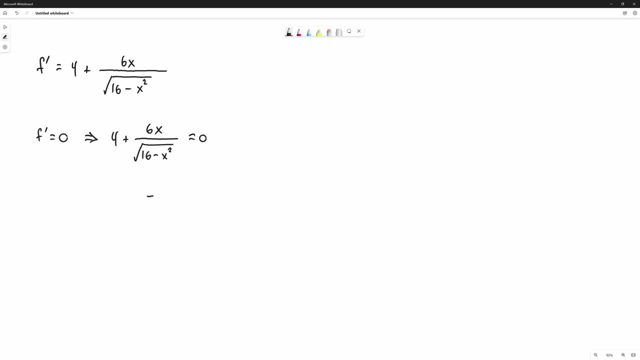 So let me go ahead and then subtract four from each side. We'll have that as six x divided by the square root. That equals negative four. Let me go ahead and get rid of fractions multiplying both sides by that square root. All right. So we're going to get rid of the fractions and the radicals. So let me go ahead and get rid of fractions multiplying both sides by that square root. So let me go ahead and get rid of fractions multiplying both sides by that square root. 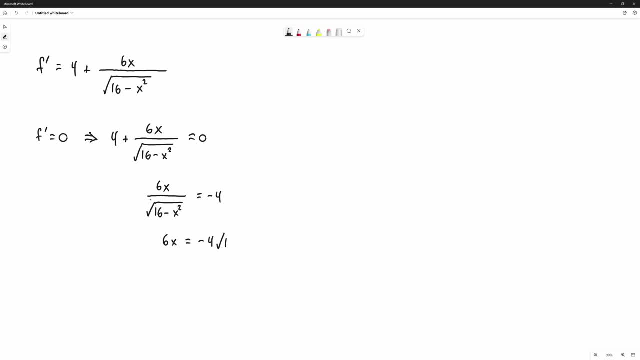 So you'll get six x equals negative four times the square root. You can simplify that a little bit, noticing there's a factor of two that you can cancel out on each side. So if you go ahead and divide each side by two, looks like you'll be left with three x, and then equals negative two times the square root. 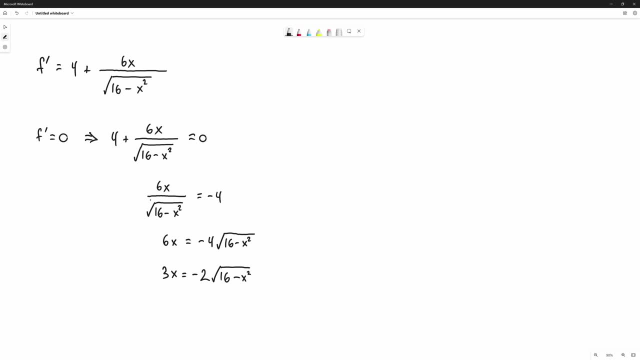 So you get zero and to get rid of the square root, we're going to go ahead and square each side. So looks like squaring to left you'll get nine x squared, And when you square the right-hand side, be careful to square both the negative two and the square root. 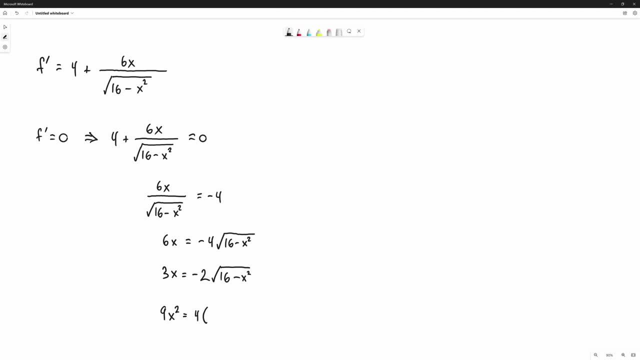 Squaring negative two, that'll turn to four And that's going to multiply sixteen minus x. squared Squaring the square root will cancel that out. All right, So we get down to this point, down to here, and it looks like, if you go ahead and distribute, looks like that's going to become. 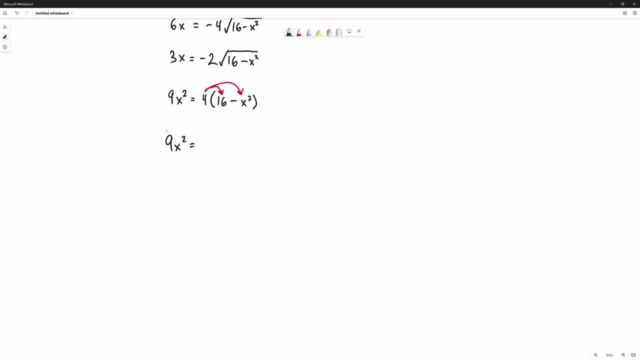 9x squared equals then 64 minus 4x squared. Now we have a quadratic equation where we can isolate x squared. I'm going to add 4x squared to each side. We'll get 13x squared equals 64.. 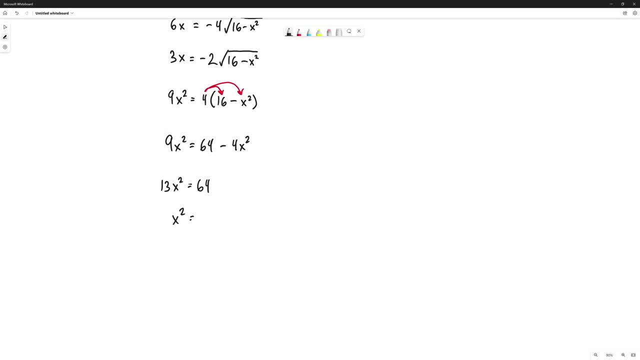 Next step: go ahead and divide by 13,, and now we can solve for x by taking a square root of 64 over 13.. Now, 13 is not a perfect square, but 64 is, so it looks like you can simplify that. 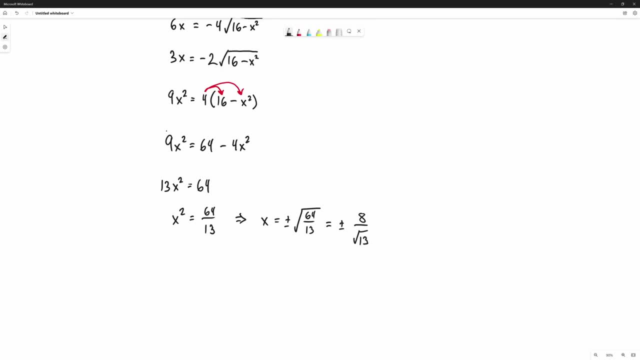 as 8. Divided by the square root of 13. And those are the critical points of the function on the boundary curve C1, the upper part of that circle. Notice that the critical points that we found have a square root in the denominator, which is okay If anyone tells you you can't have square roots. 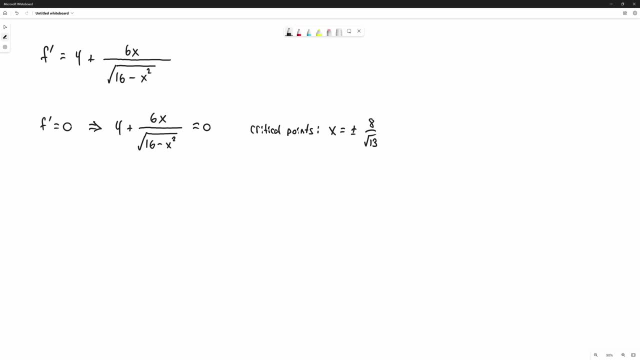 in the denominator. they're lying and they don't know what they're talking about. So we're going to leave that as plus or minus 8 divided by square root of 13.. But important in this example is the first. the square root minus 5 is equal to the middle. 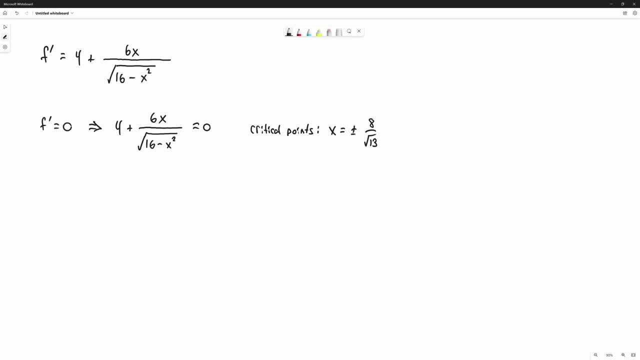 heart of this讲ticket. The lived mark is my square root of 5, and then there are five times the square root of 5. successful Quad antennas don't work, So I make theumber and square root When it comes to ALT, plus 1 times the square root of 4, you can quantize it- and 2 plus 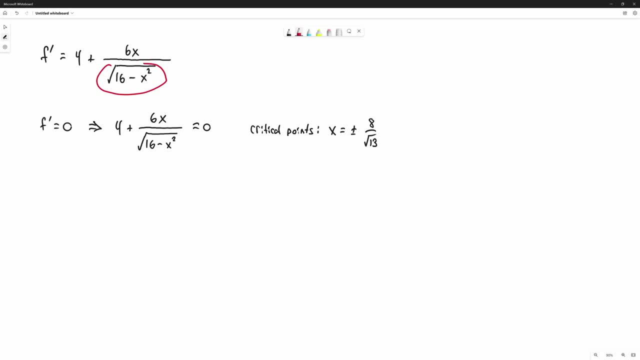 13.. You can rationalize it if you want. I'm not going to Now. what we're going to notice is that the denominator of the derivative, that is a possibility of also becoming 0. And that means we might have the possibility of getting critical points where the first 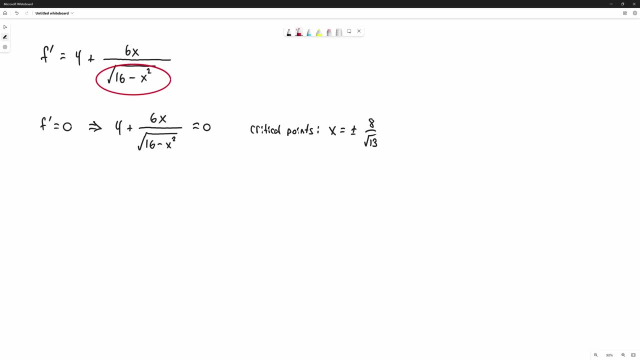 derivative is undefined. Now that denominator is going to become 0 when x is 4 and negative 4.. And that is the interval that we're considering. The left end point of the interval should also be equal to the values of x point of the interval for x values. basically, you think of the circular region that was 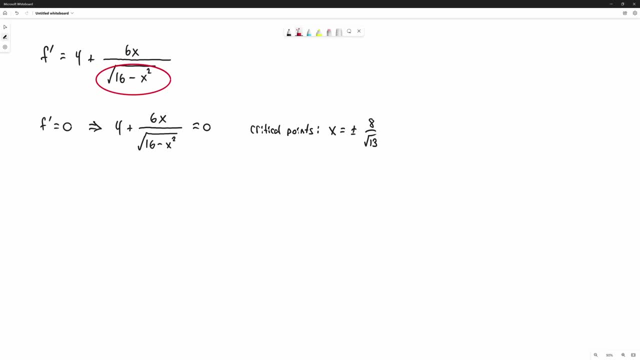 a circular region or disc of radius 4,. so the left end point of our interval for x is negative 4,. the right end point of our interval for x is positive 4, so the values that make this derivative undefined, well, they're also the values of our interval that we're considering. 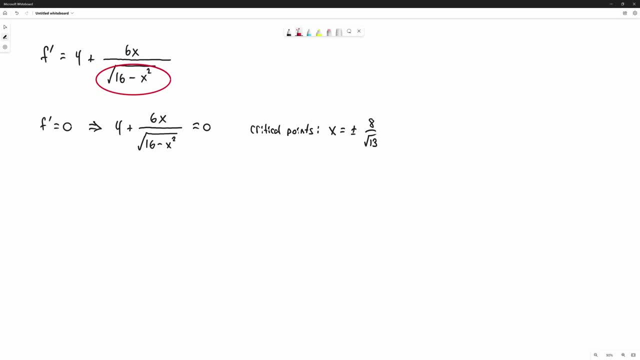 here, so we don't need to duplicate that. so what we're going to do is check the value of the function on curve 1, the upper boundary curve at the critical points and the end points negative 4 and 4.. 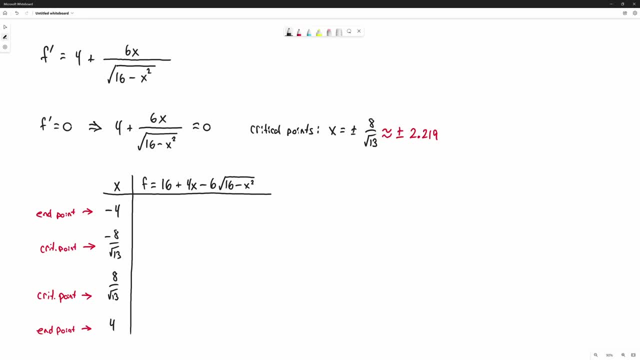 Two of these x values of interest are going to be easy to plug in: negative 4 and positive 4, that's going to make that square root expression the square root of 16 minus x squared. that's going to evaluate to 0 when x is negative 4 and 4, so let's do the easy values first. 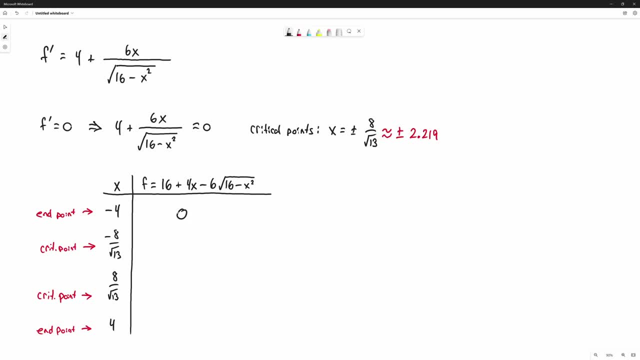 plug in the value of the function on curve 1, the upper boundary curve at the critical point, and plug in negative 4, that restricted function value on curve 1, that's going to evaluate to 0, and plug in positive 4, and we'll get 32.. 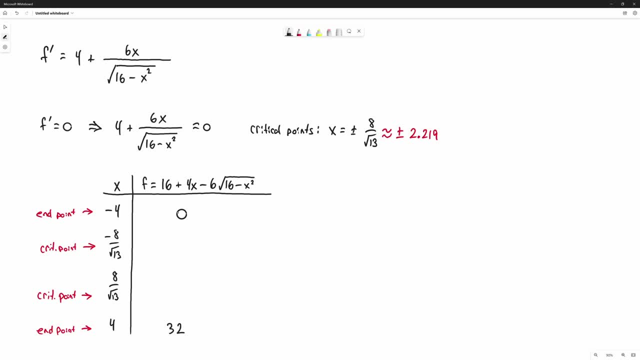 We're going to work through the next one, plugging in the critical point: negative 8 divided by square root of 13, we'll get an exact value which you can also approximate as a decimal value. notice there: the critical points are approximately plus and minus. 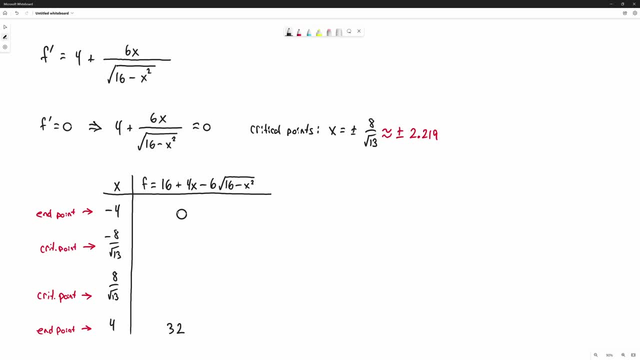 2.219, and that's between negative 4 and 4.. So let's slog through, plugging in x as negative 8, divided by square root of 13, to our restricted function. All right, we're going to take the restricted function. this was plugging in the curve, for. 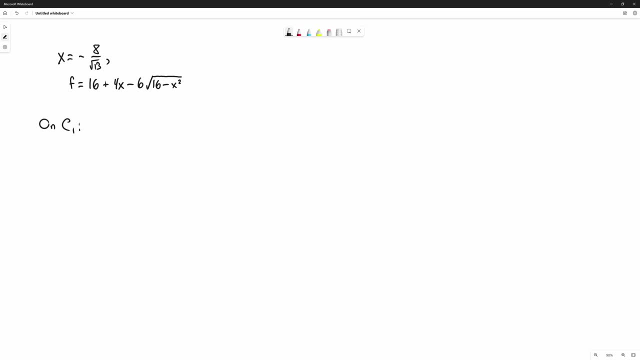 c1, y as the positive square root of 16 minus x squared. we're going to plug in the critical point: negative 8.. That's a square root of 6, that's a negative 0. That's a critical point. we're going to plug in the critical point: negative 8 divided by: 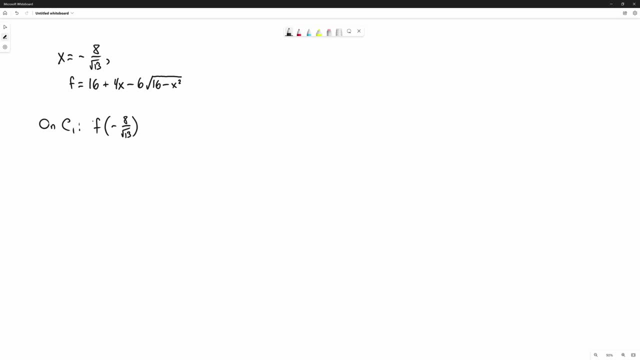 square root of 13, and simplify that completely. All right, so if we go ahead and take our time doing that, looks like we'll get 16 plus 4 times negative, 8 over square root of 13, and then minus 6 times the square root of. 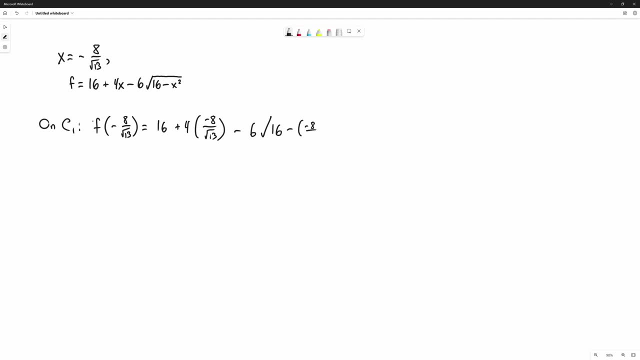 16 minus negative 8 over square root of 12.. That's the key. So I get 16, and I need to multiply that by that and that's going to be negative 8 divided by the square root of 13.. 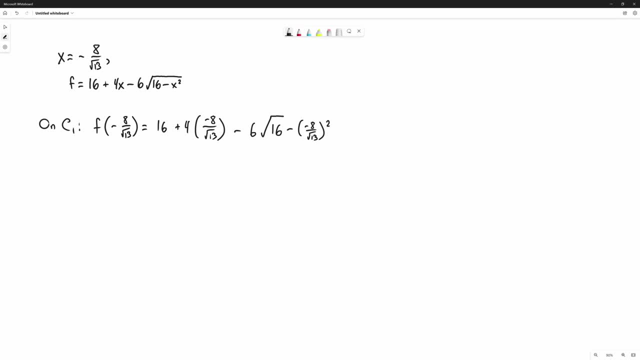 over square root of 13,. all that squared, All right. if we go ahead and take our time, we're going to get 16,, 4, and negative 8.. So I can write that as 32 over square root of 13.. 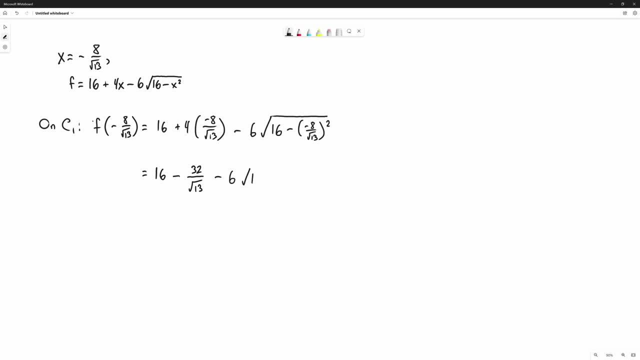 We're going to have the minus 6 out front And then inside notice. the square is going to knock out the negative, but we still have the subtraction sign there. 8 squared that's going to come out to be 64.. 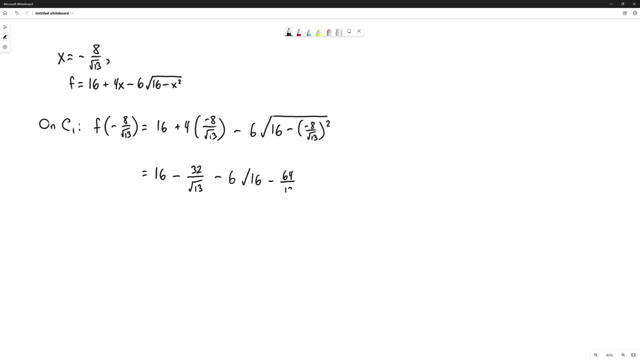 And then squaring the square root in the denominator, that'll just become 13.. All right, now with a little bit of tedious arithmetic. here you can use a common denominator and simplify that, And that should come out 16 minus 64 over 13,. that should come out to 144 over 13.. 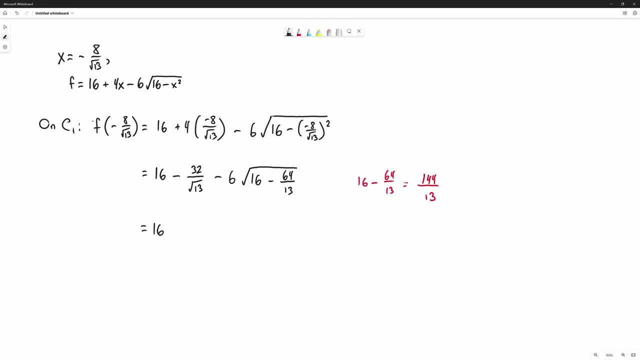 So here it looks like we get the value of our restricted function at the critical point. We're simplifying that slowly but surely. All right, that square root expression evaluated to the square root of 144 over 13. And you might recognize 144, that is a perfect square. 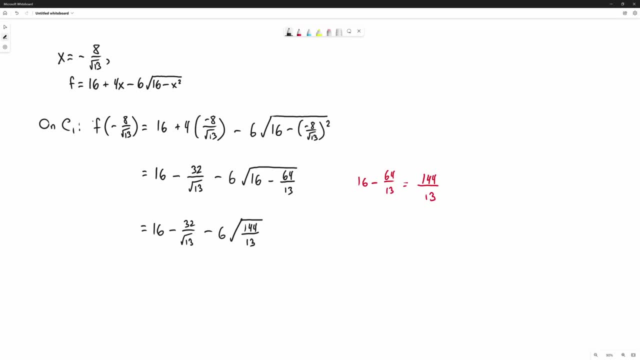 So that's going to simplify to just 12.. So it looks like here we get 16 minus 32 over square root of 13. And then minus 6.. Square root of 144 is 12.. Don't forget to take the square root of the denominator as well. 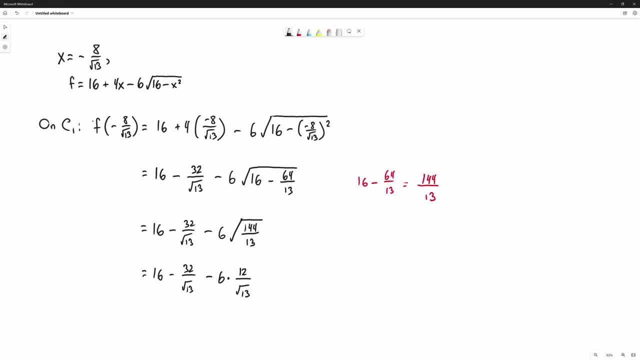 Giving you another denominator of square root of 13.. All right, now, if you go ahead and simplify this notice here, you can basically write this all as a fraction over square root of 13.. You have negative 6 times 12.. That'll become negative 72.. 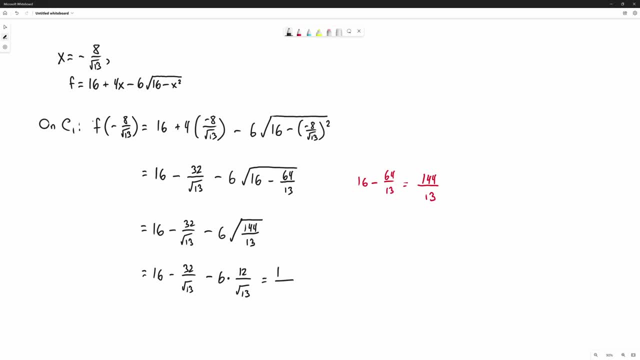 So if you were to write this all with a common denominator, the common denominator being square root of 13,- we get kind of an unpleasant looking exact value here And it looks like here we all have the same denominator for those fractions And we have negative 32 minus 72.. 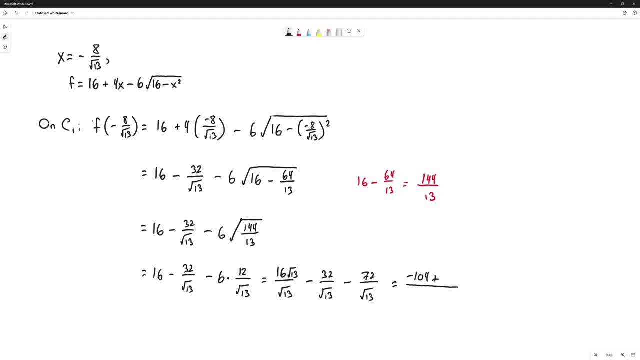 That comes out to negative 104.. And then plus 16.. Square root of 13.. All divided by square root of 13.. And that is the exact value of the restricted function on curve 1 at the one critical point: negative 8 divided by square root of 13.. 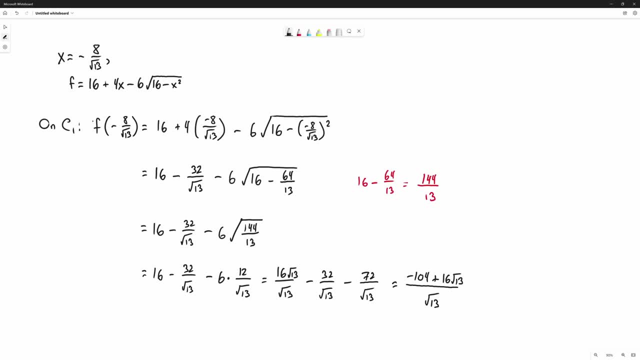 Now, just for reference, to do the comparison, you can plug that into a calculator And you'll get that this approximately evaluates to negative 12.. And you'll get that this approximately evaluates to negative 12.. 0.844.. All right, we're going to write it in the exact value. 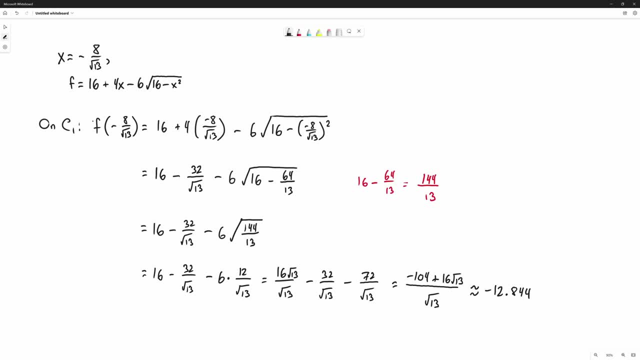 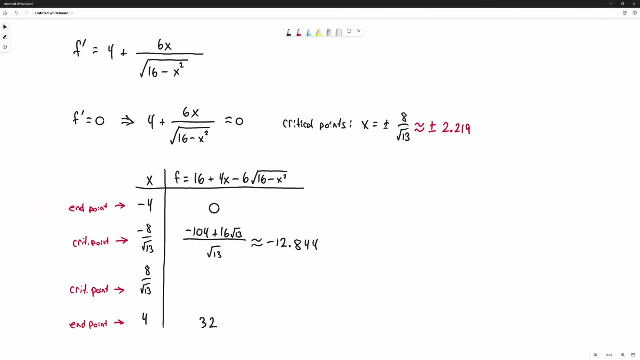 but in the table we'll put both, just to make the comparison a little bit easier. So let's go back to our table of values from above, Plugging in the other critical point: positive 8 divided by square root of 13.. That is equally tedious. 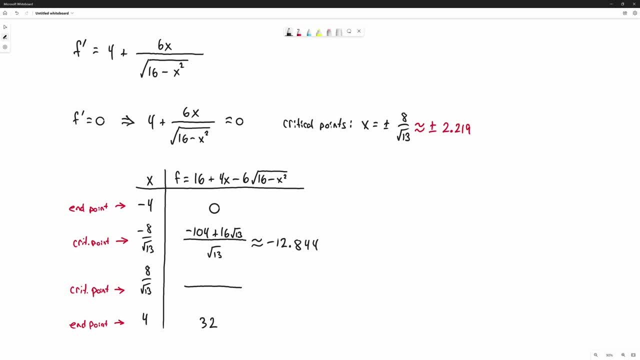 And if you go through pretty much the same work, a lot of the steps give the same simplification for the numerical values. What you're going to get instead, and take your time with this, you'll get the exact value as negative 40. 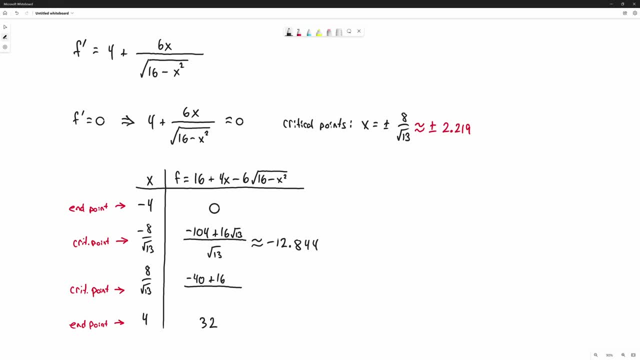 plus 16 times square root of 13, all over square root of 13.. And again, just take your time with that. It's exactly the same as what we did with plugging in negative 8 divided by square root of 13.. 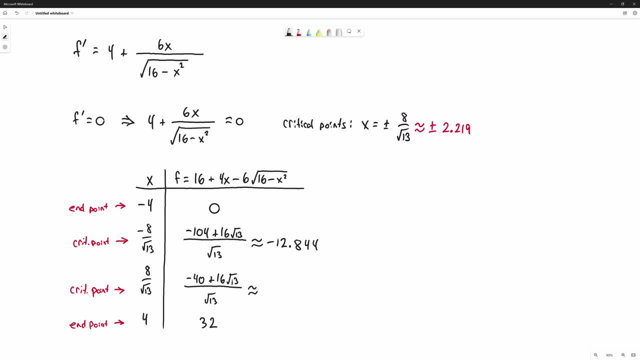 And if you go ahead and get an approximate decimal value for this critical point, that comes out to about 4.906.. All right, and these are the values of interest of our restricted function on curve 1, the upper part of that circle. 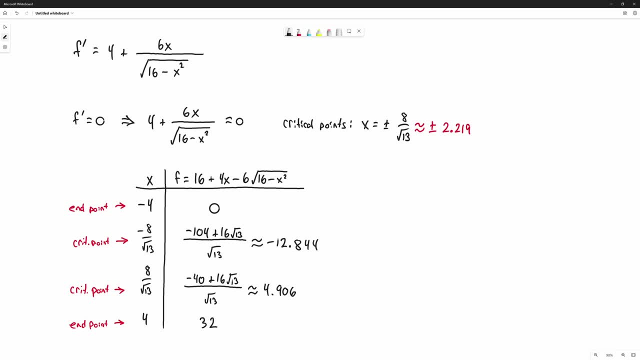 Let's go ahead and check for the absolute max and min values, the values of interest, on the bottom portion, curve 2.. The only difference with the work for checking the values of interest is that the values of the function on curve 2,. 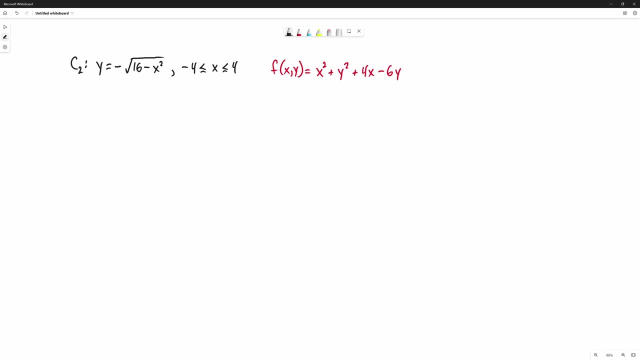 the bottom portion is that the y, the function just has an extra negative there. So we're going to plug in y as negative, the square root of 16 minus x squared, And what we get for the function now just of one variable. 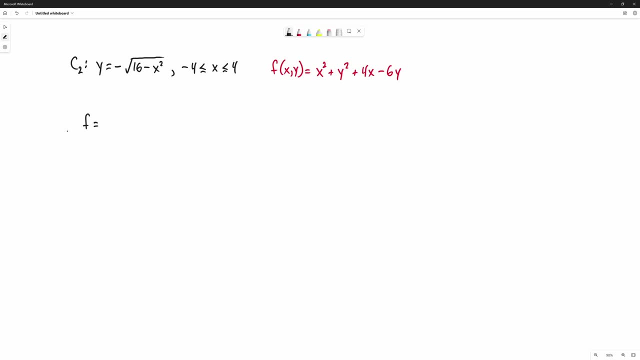 because we're restricting it to curve 2, it's going to become x squared. We're going to go ahead and square negative the square root of 16 minus x squared. That's all squared. We have plus 4x And then minus 6.. 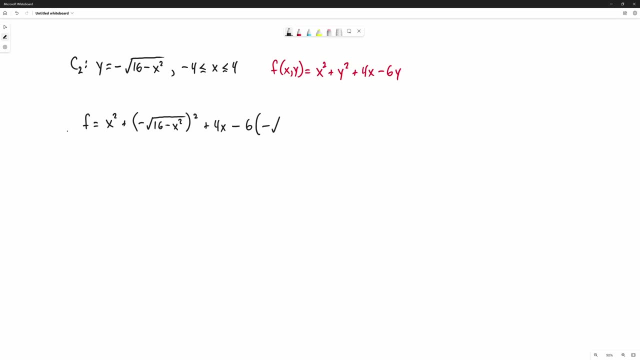 And be careful there- We're going to get a negative that cancels. We're replacing y with negative- the square root of 16 minus x squared- And that is really the only difference we're going to get, instead of a negative from before. 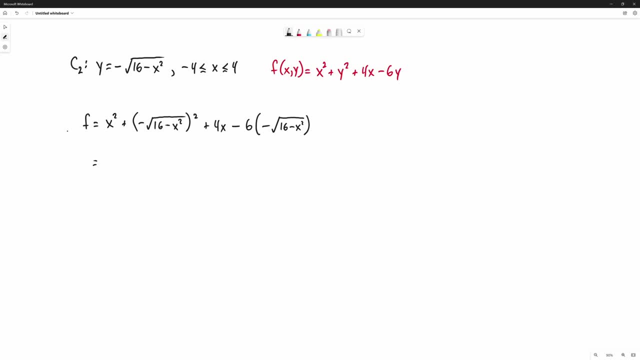 a positive from before. So we're going to get a positive from before and we're going to get a negative from before and we're going to get a negative from before in front of 6.. So if we simplify this, it's like we'll have x squared. 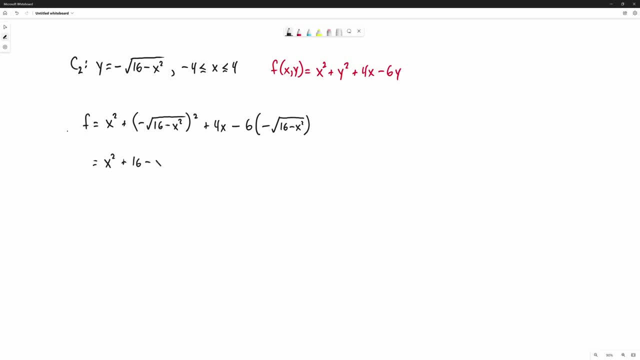 and then plus 16 minus x squared plus 4x, but now plus 6 times the square root of 16 minus x squared. And from there, notice, you can again simplify the x squareds. cancel out and this simplifies to just 16 plus 4x, which we had before, but now plus. 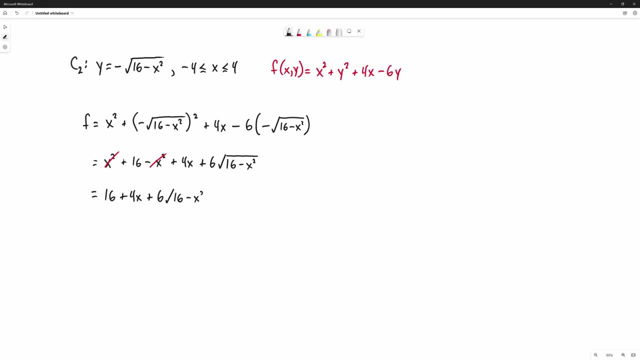 6 times 16 minus x, squared. all right, and from here it's all the same. work from what we did before on checking the boundary values on curve one. if you go ahead and calculate the derivative the same as we did for curve one, you'll find that you eventually get the same critical points for this restricted function. 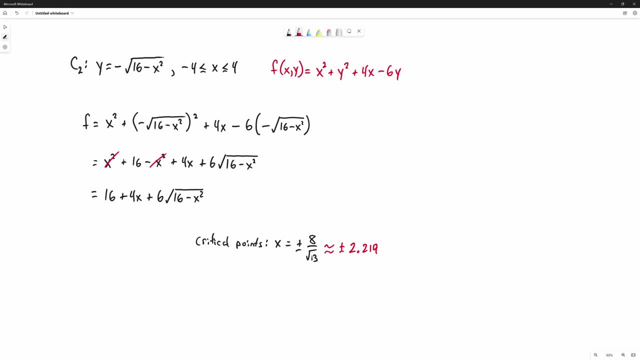 on curve two, again the critical points work out to positive and negative. eight divided by square root of thirteen, and the rest of the work is again virtually identical, just with some subtle changes in one or two signs here and there. so let's go ahead and check the values of interest. 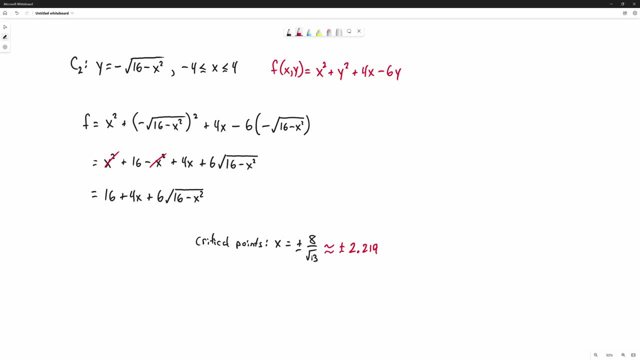 our function at these two critical points and the end points of our interval here. negative four and four. now that we have the critical points, we can check the values of the restricted function on curve two at the end points and critical points. all the work is identical to before. negative four. 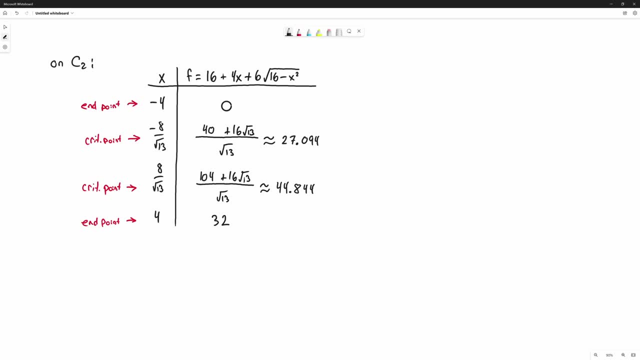 when you plug that in for x there to our restricted function, that's going to evaluate to zero. and when you plug in four, well, that's going to evaluate to 32.. plugging in the critical points, positive and negative, 8 divided by square root of 13, again that work is very similar to what we did earlier in the video. 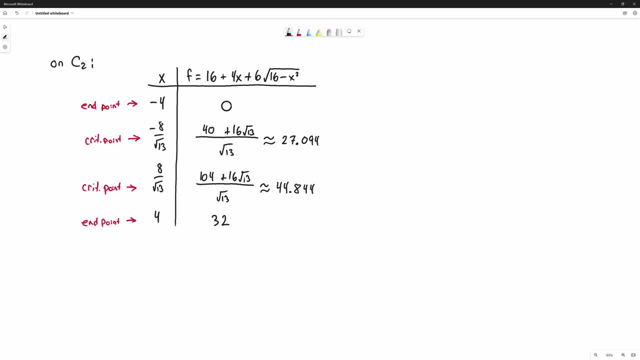 so take your time with that and you'll get similar fractions: 40 plus 16 times square root of 13, all over square root of 13, and then for the positive critical point, you get a 104 instead of the 40 there. all right, if you write those as their approximate. 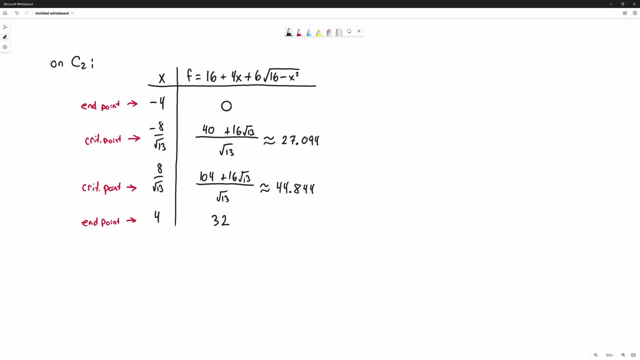 decimal values, those values at the critical points come out to about 27.094 and 44.844. at this point. we have all the calculations done. we just need to compare all of the values of interest, the values of our function at the critical point, the values of the function on curve one. 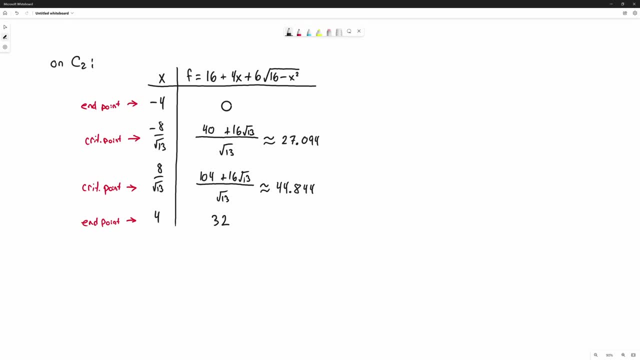 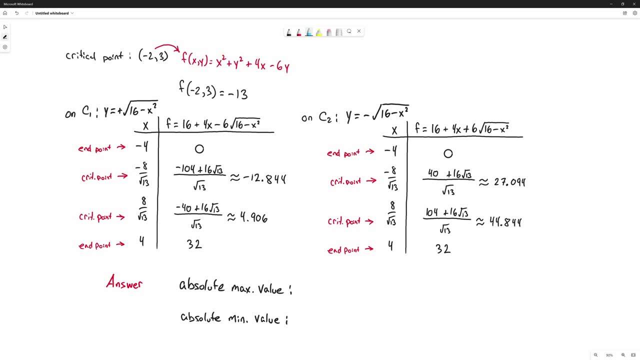 and the values of the function on curve two. let's put that all on screen together. at this point, we just need to compare values. so let's start by looking for the biggest function value, and that looks like that's over there: the absolute max value, the biggest function value that we get. 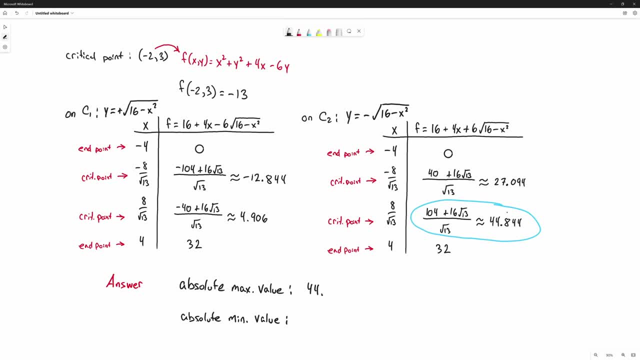 this is on curve two, the bottom portion of the region, or bottom boundary curve, and that's 44.8, four, four, and if you now look for the smallest value, looks like we get that here at the critical point and that comes out to negative 13.. and for this problem, that is the 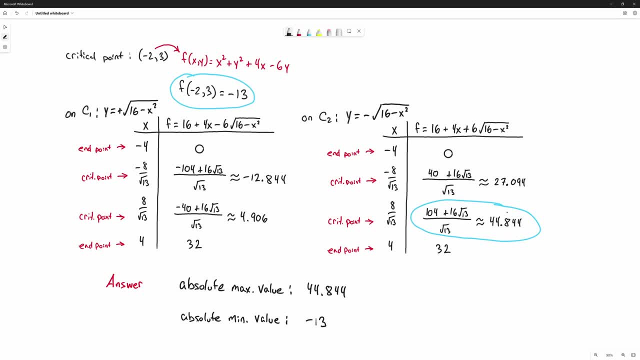 answer. the absolute max value is 44.844. the absolute min value is negative 13.. now, for some of your courses you might want to determine. those are the values, but where do they occur? and if we take a look at the max value, that's an x value.